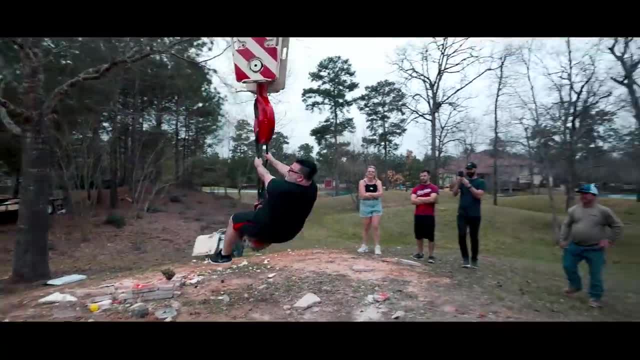 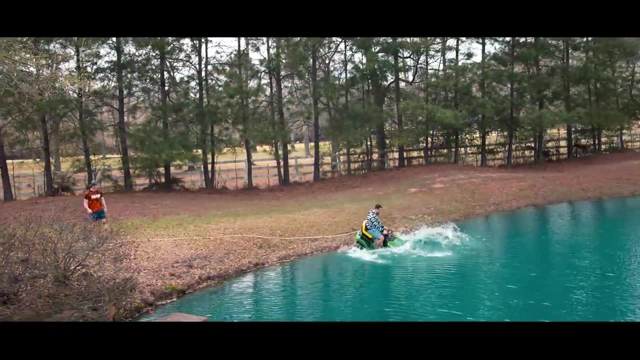 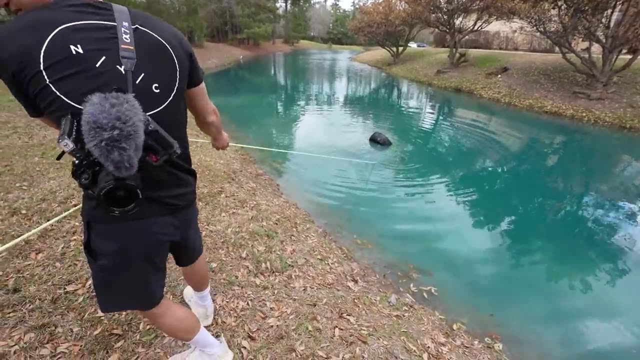 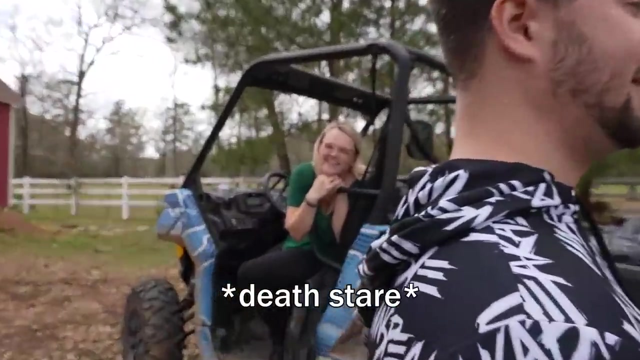 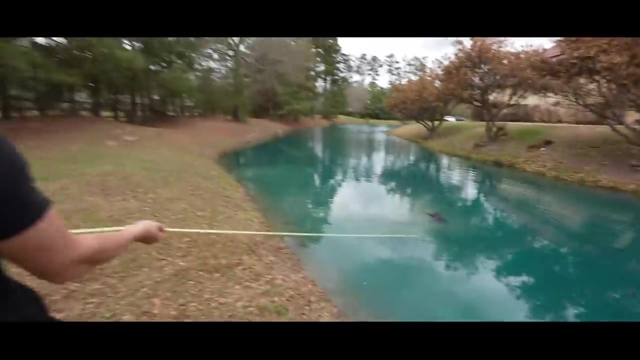 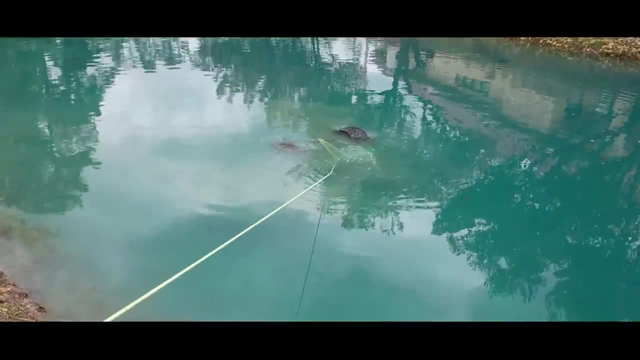 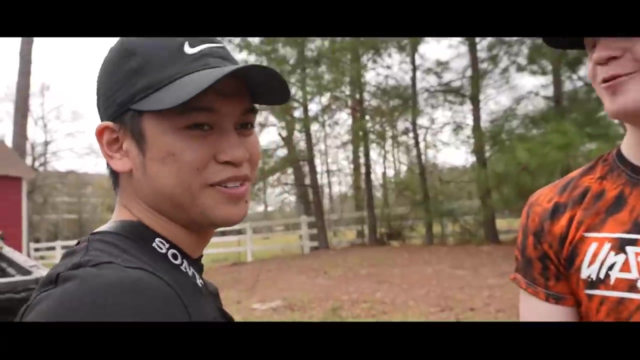 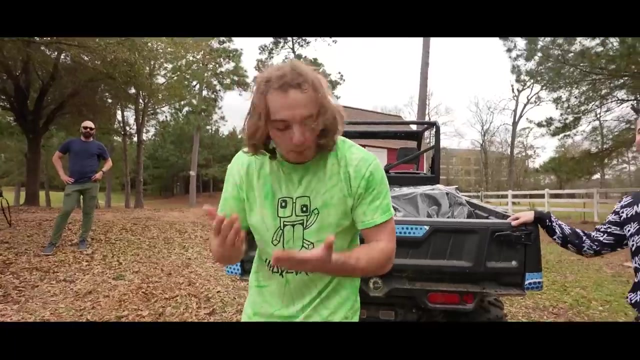 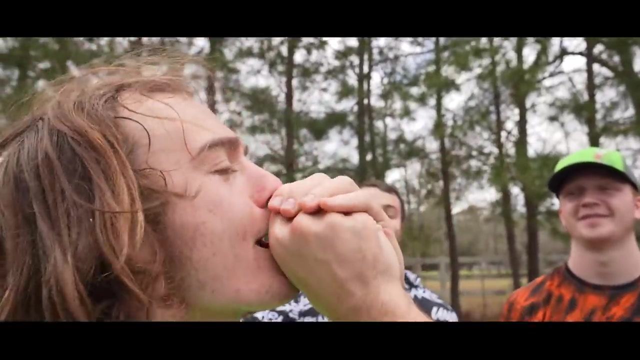 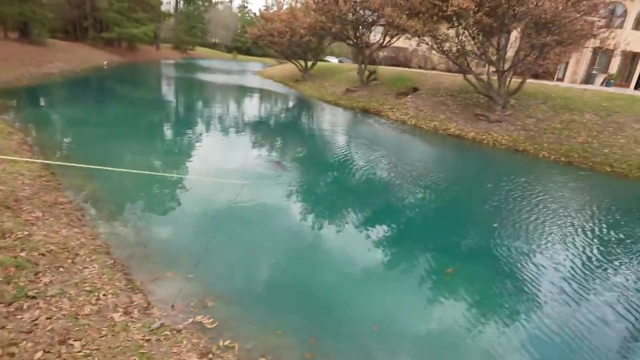 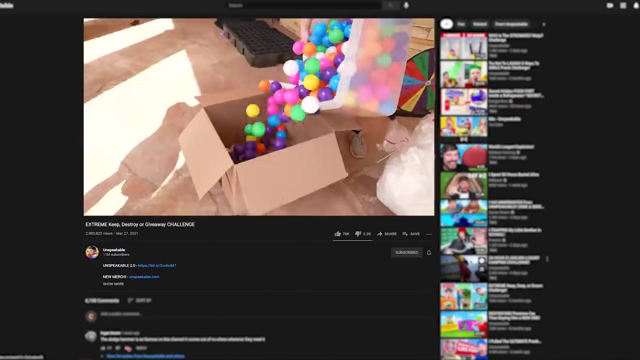 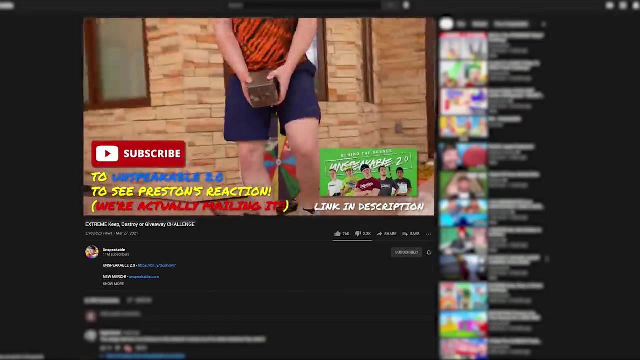 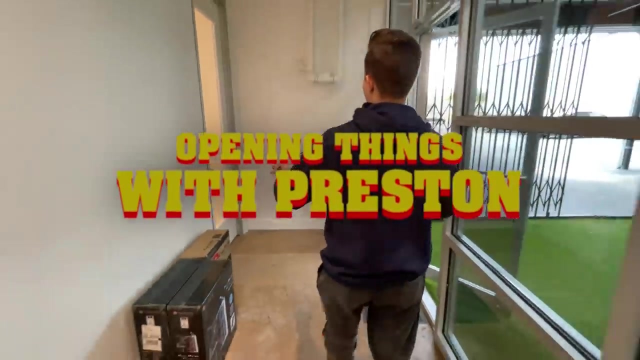 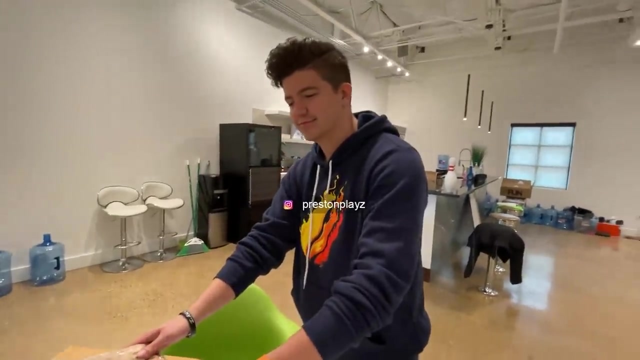 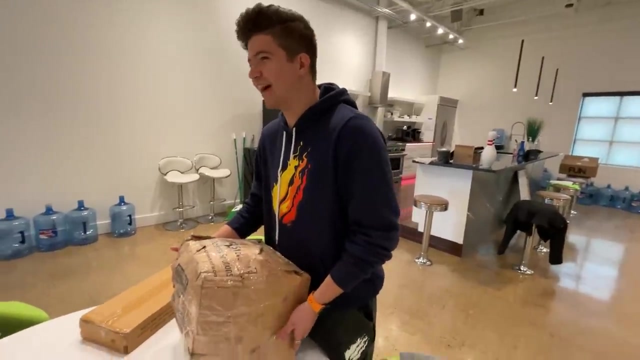 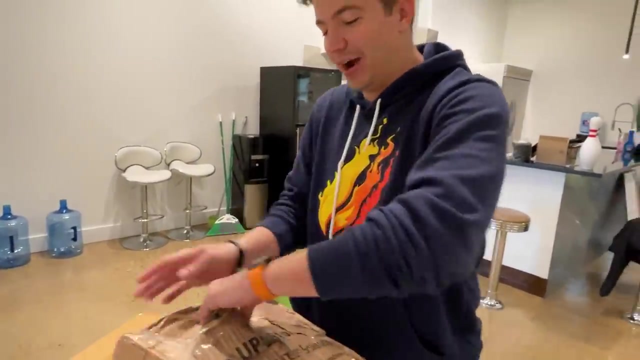 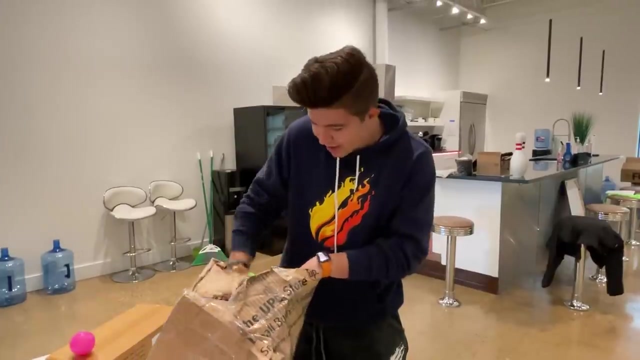 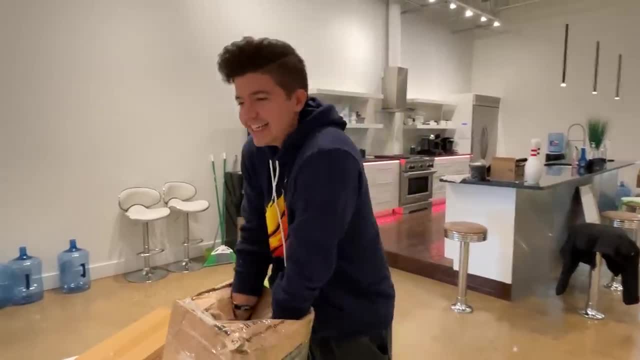 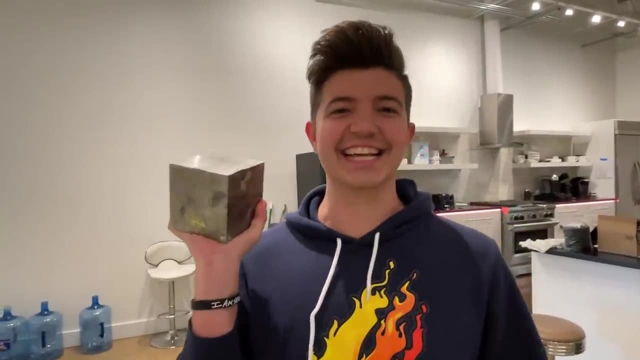 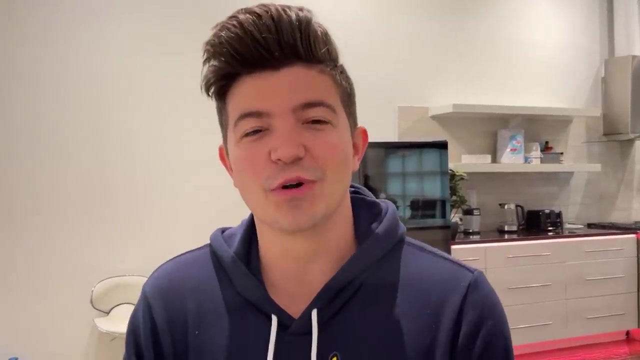 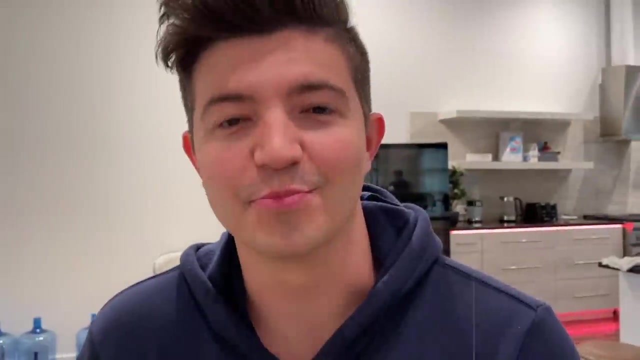 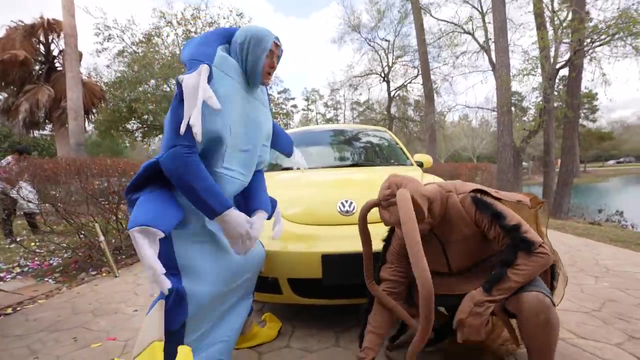 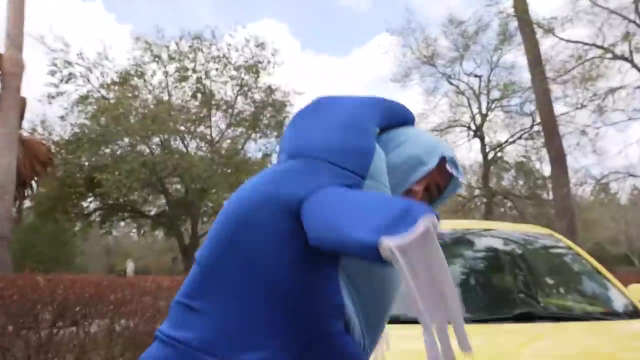 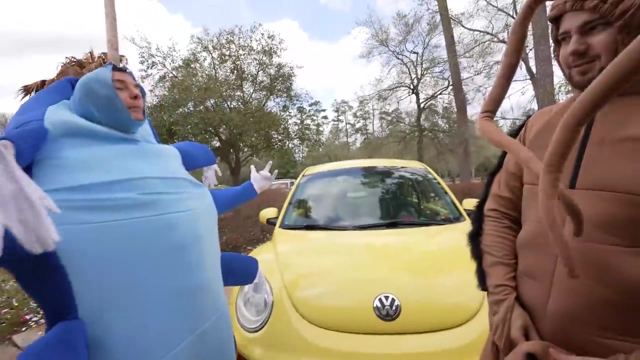 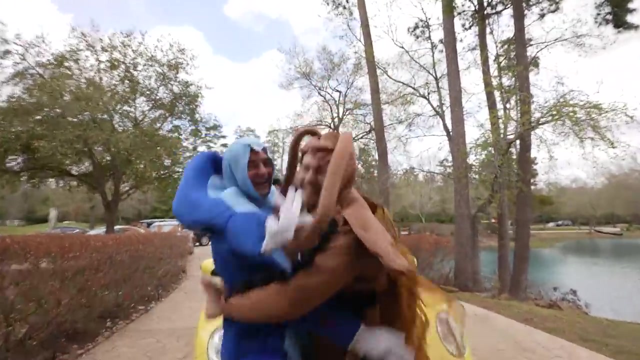 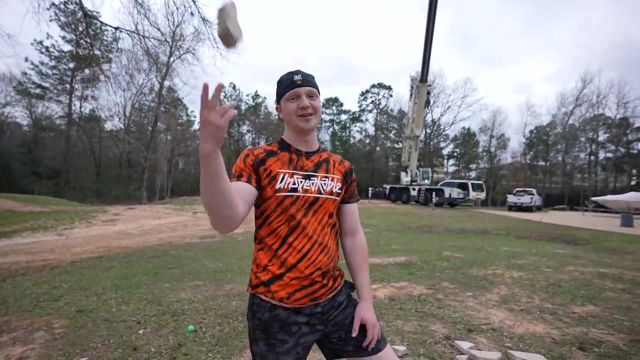 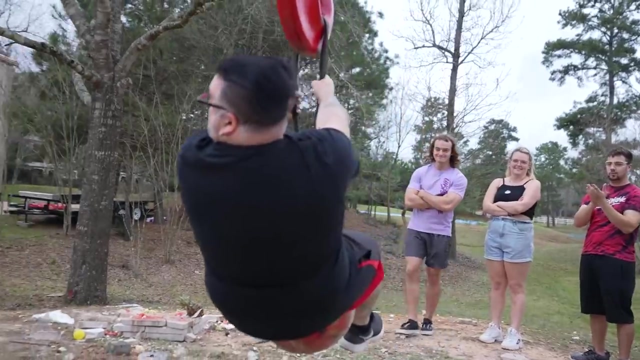 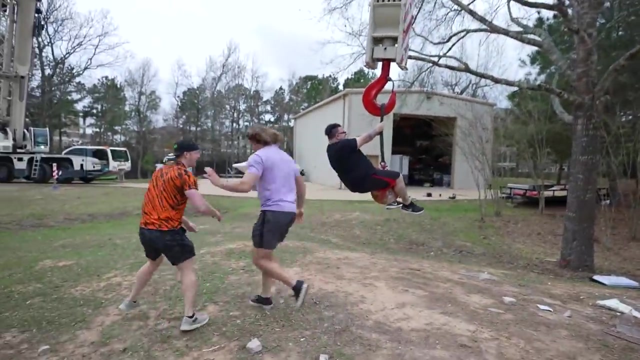 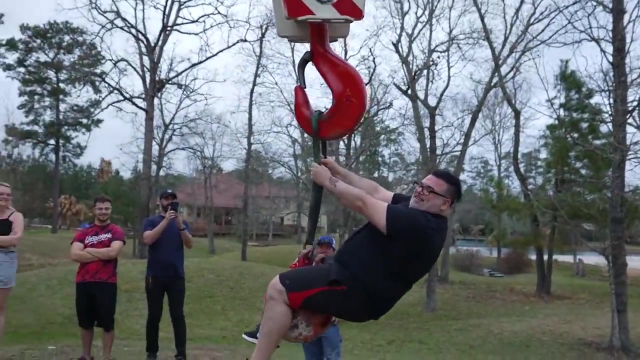 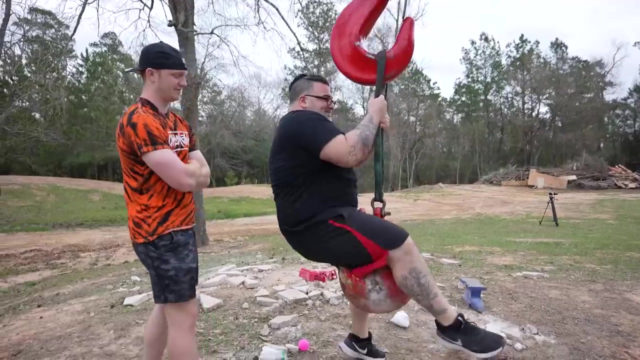 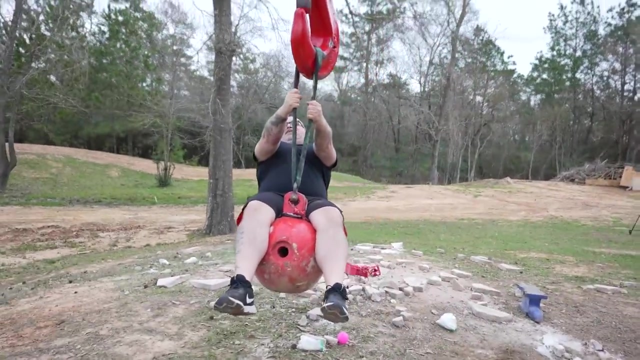 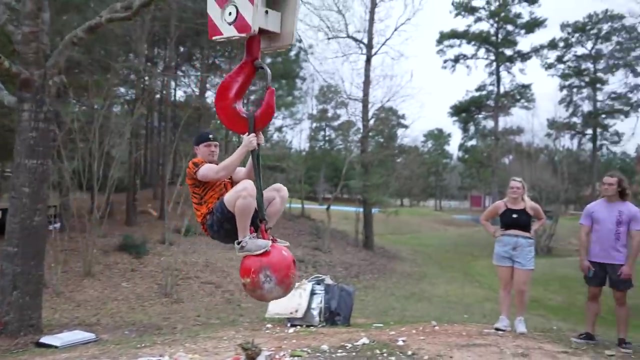 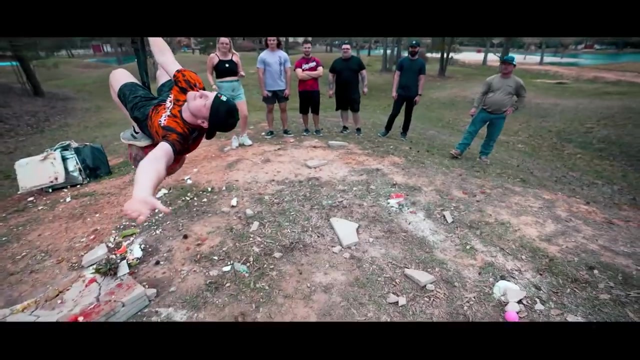 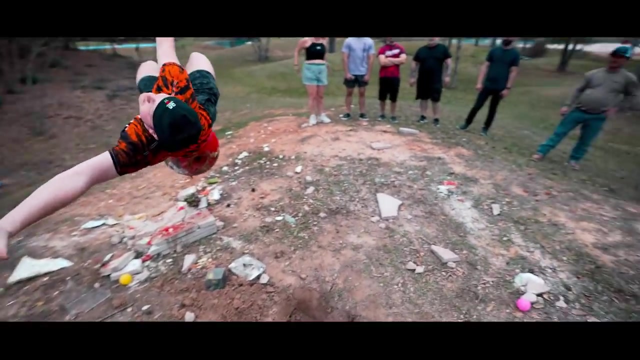 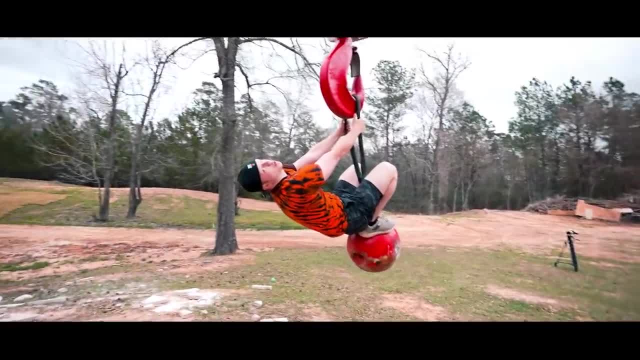 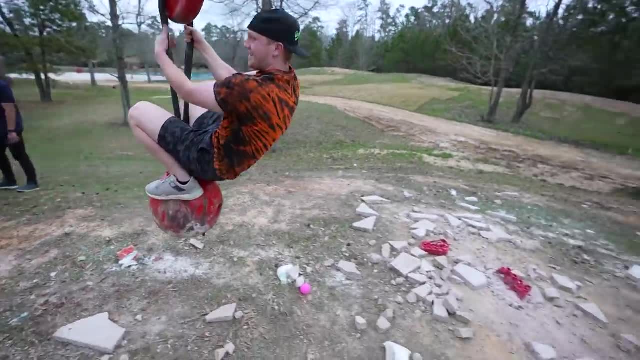 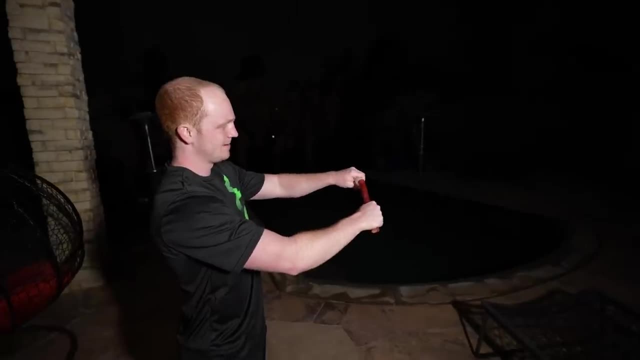 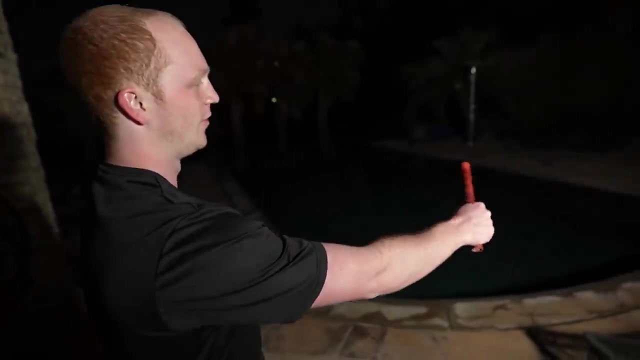 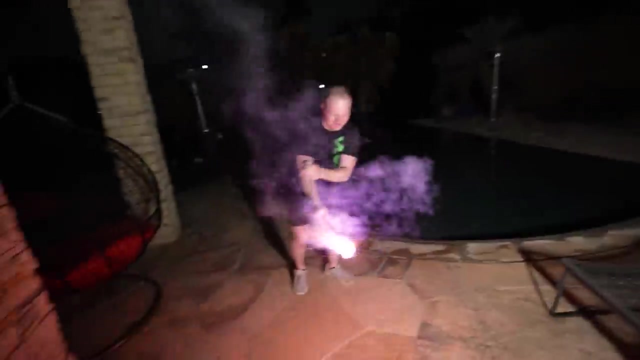 Thank you for watching. Please subscribe, like and share. I won't deny it. You know you make me feel so alive. I wanna stay with you, baby, I'm scared The fire- Oh, it's hot, It's burning me. So apparently this thing can go underwater. 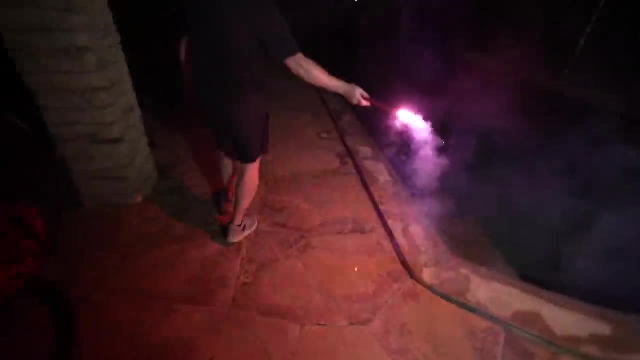 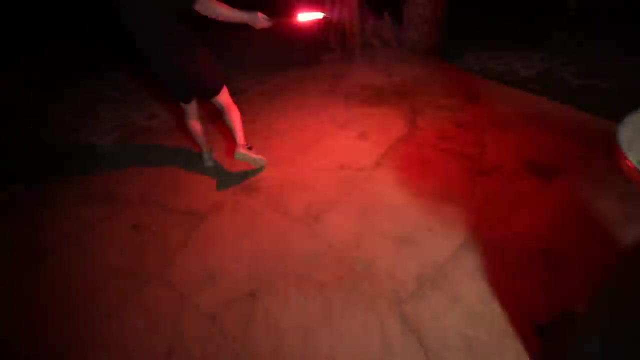 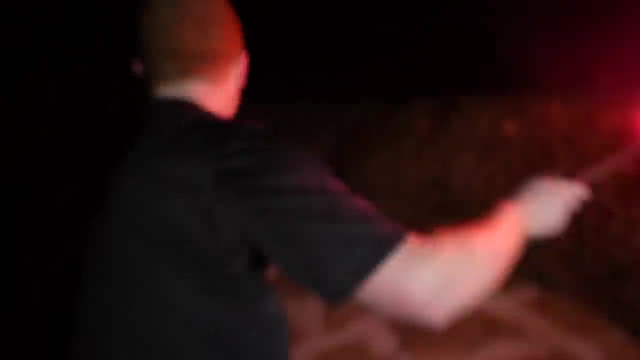 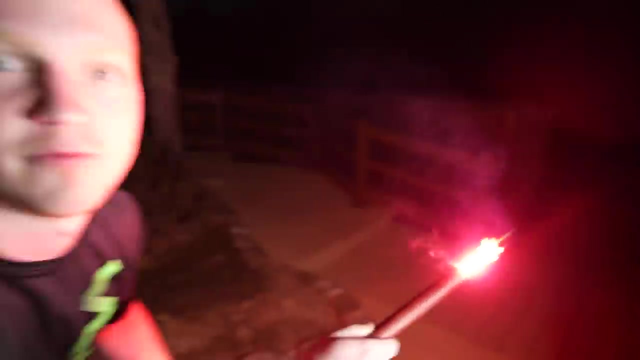 So let's see, follow me, Wait, I don't wanna follow you. You're dropping like lava. It's on my toe Point in another direction. Ta, ta, ta, Wait Here in the wild. Would you look at that over there? I see nothing, Right, there's nothing. 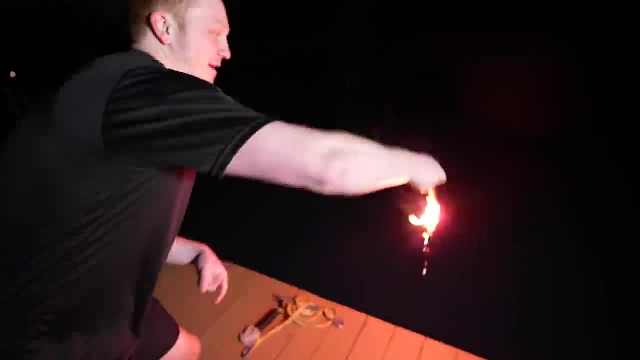 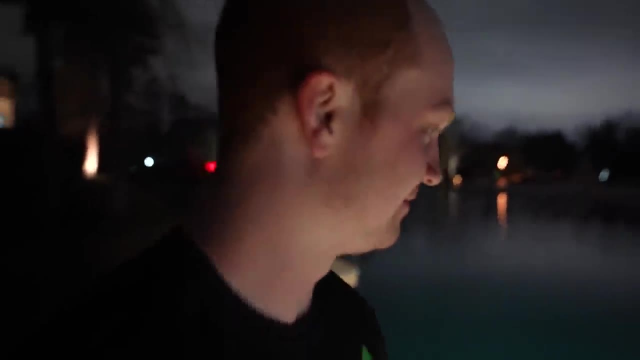 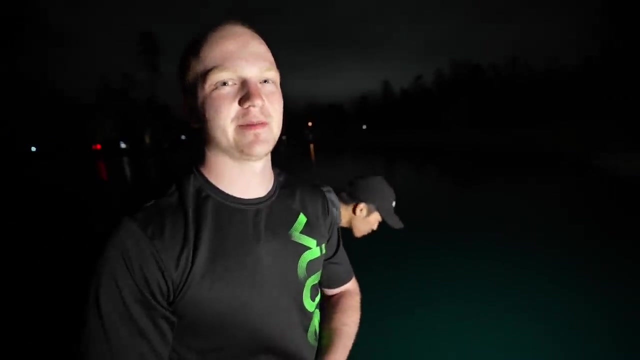 I keep stepping on it. It's on fire. It's supposed to stay on, Is it? I don't know if it's supposed to stay on. It's supposed to be like a waterproof kind of thing, But it just kind of What if we fix you in? 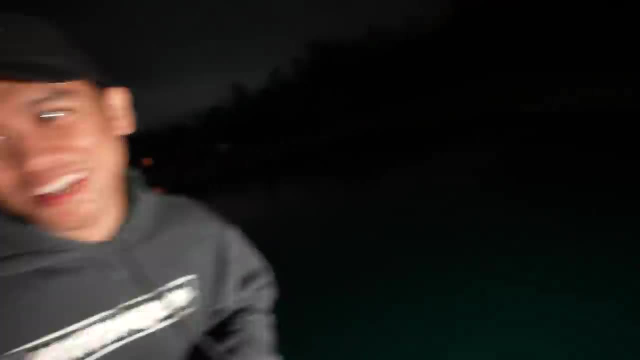 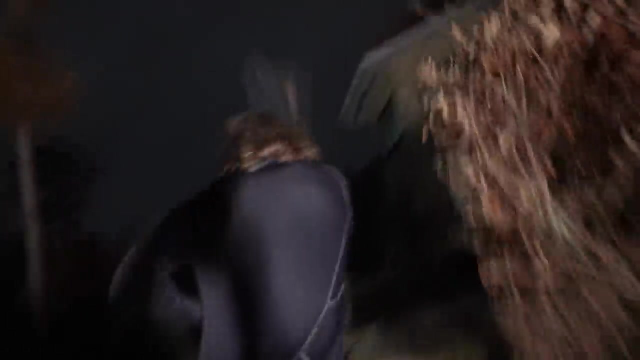 I'll take you in with me. I dare you to do it. Nah, we didn't sign anything. Come here. come here. What did you say? Is that a net? I pulled it out my wetsuit. Go catch him. Come here, Pokemon. 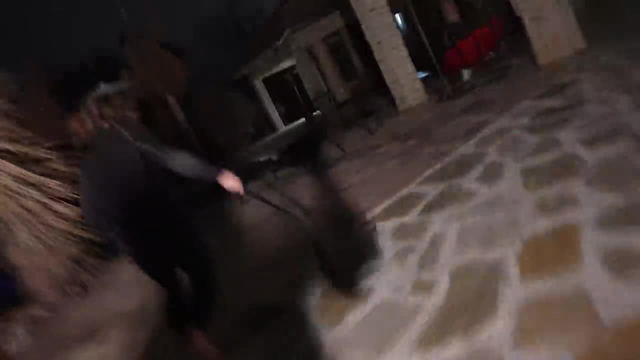 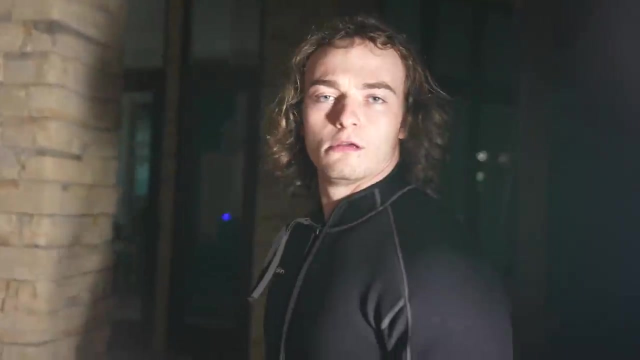 Catch that Pokemon, Catch that Pokemon. Hurry, get him. He's in the chair. I need my Pokeball. I mean, he's in his Pokeball, it's his masterbook. Uh, he already got caught. that's why. Hey, the other side of the ball is open, he can get out. 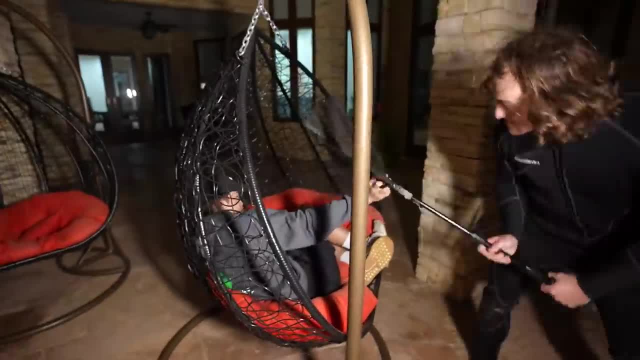 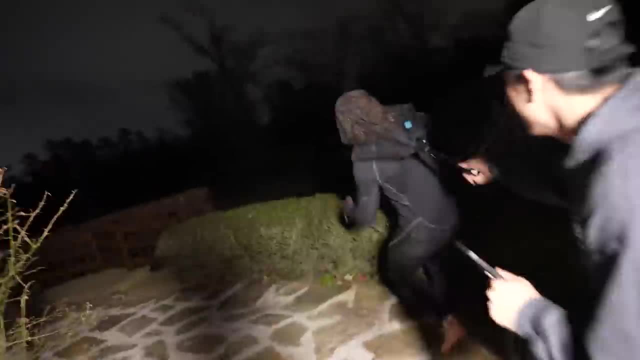 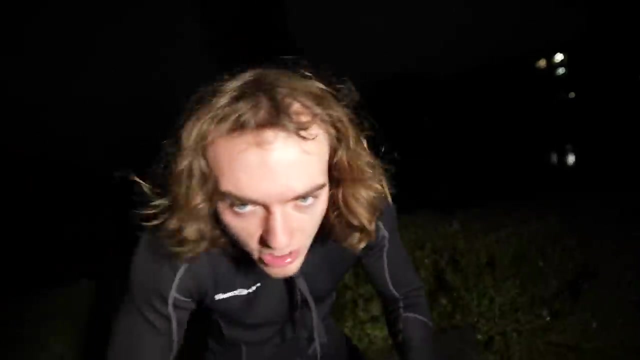 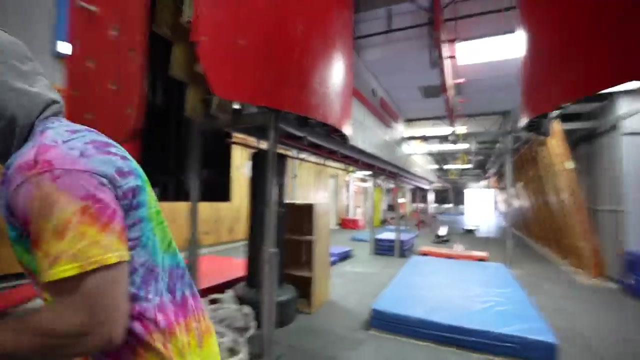 No, You're mine, boy, Come here. No, Accept me as your trainee. I'm your trainee, Pikachu, I made my Pokeball, Got your ball. Ow, I came in like a robot. It's pretty sad. It's a creeper. 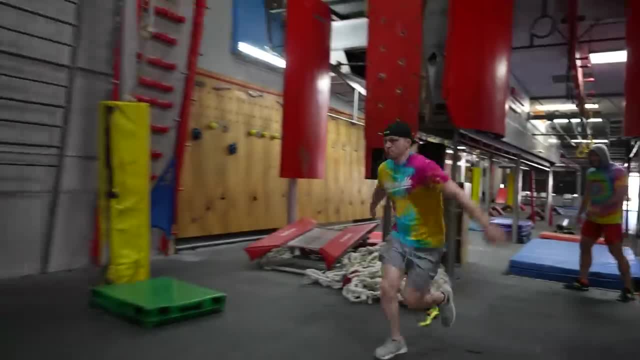 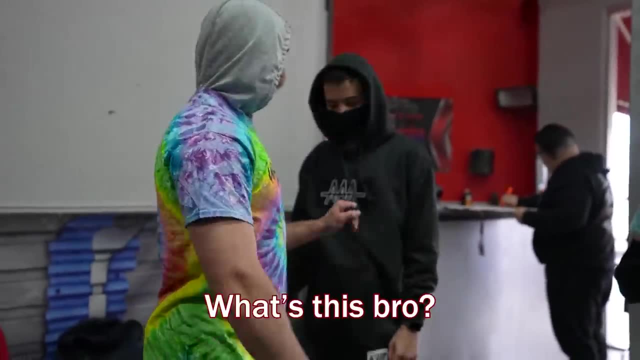 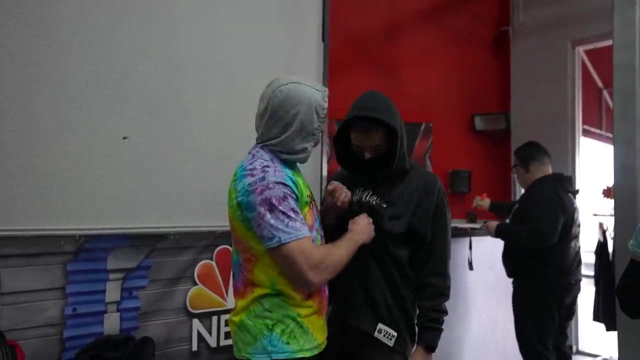 I landed in my haystack. Have you seen this man, Dude? this is gonna happen, Did I? What's this, bro? What's this? Free merch? What's this? Is that Team Raw merch? I'm not a traitor, I swear. 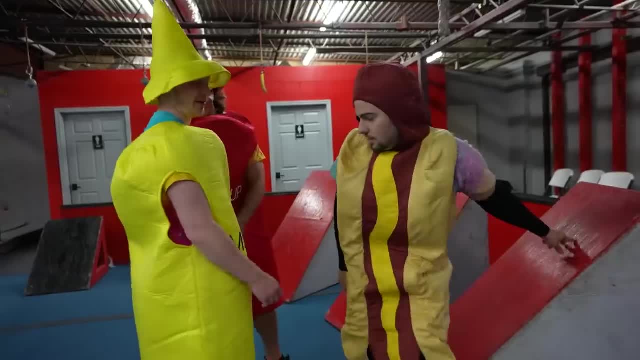 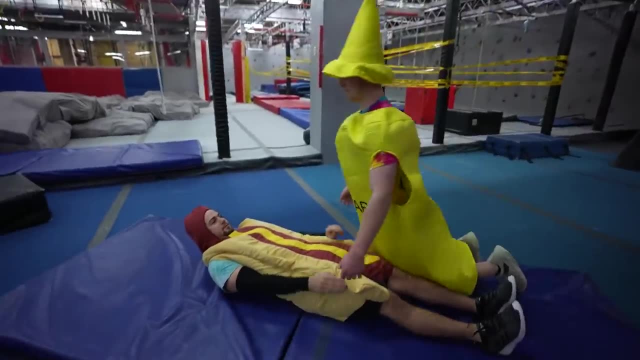 Filing Chapter 7 bankruptcy. Look at this glizzy. I don't want ketchup, I want mustard. Come on, Sauce me up, dude. Sauce me up, dude. Oh, that's too much mustard. Yeah, you want some ketchup? 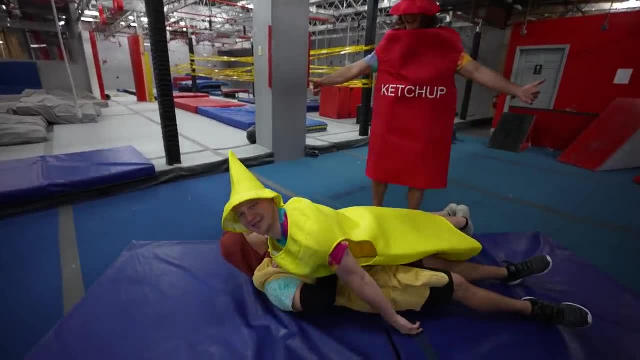 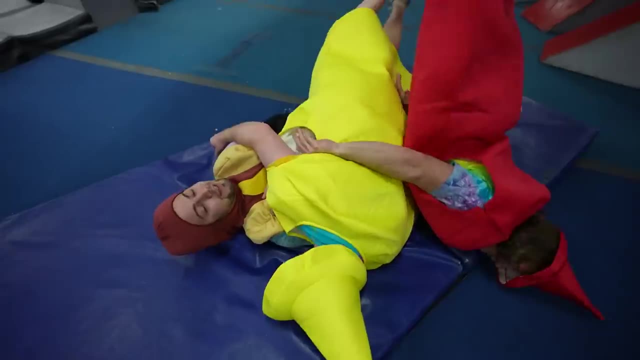 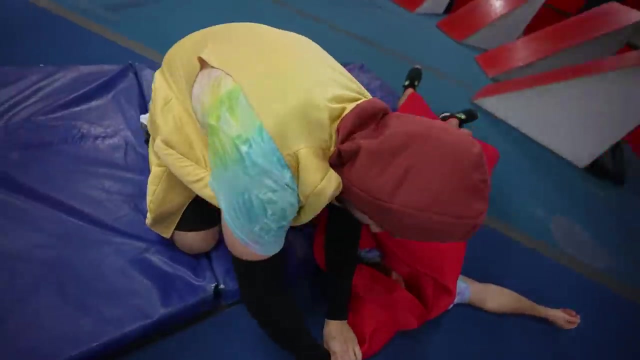 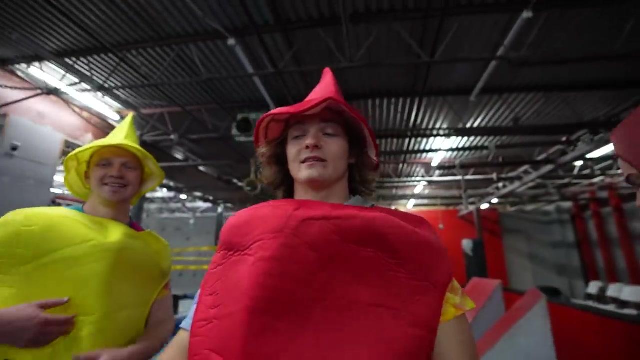 No, Yeah, I don't like ketchup. Maybe I want some ketchup, Ketchup, Ketchup, Bro. you squished my bun. Your mustard is expired, bro. You ready to get ketchup? Sorry. So this dad, tomato and his son, was going on a walk. 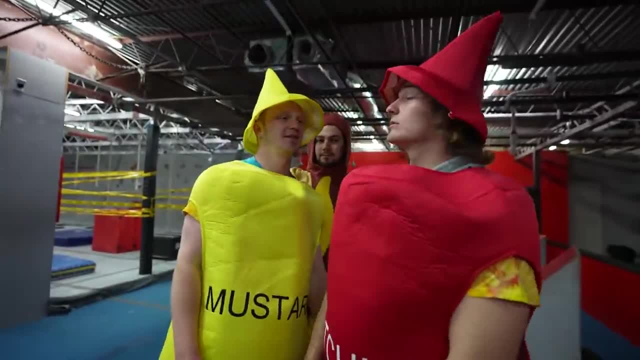 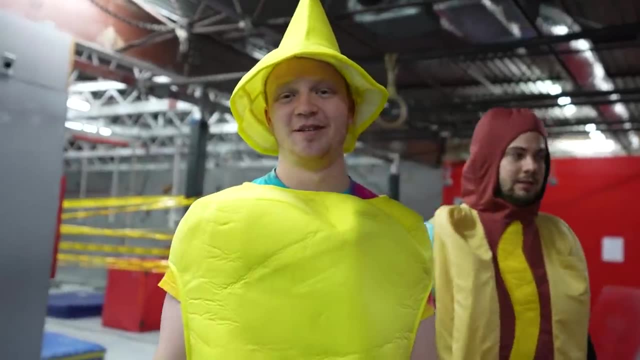 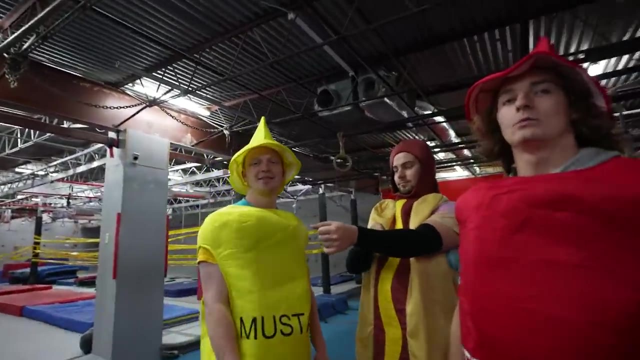 And his son started falling behind. The dad looked at him and goes: Ketchup, I'm just mustard, there's no jokes. I mustered to ask you a question. Alright, Jordan, here's the deal: If you can hang on this bar for 100 seconds. 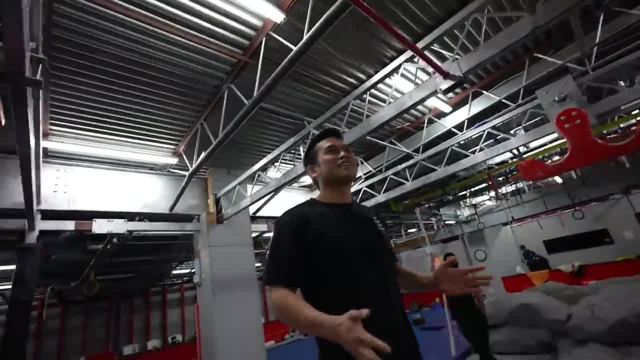 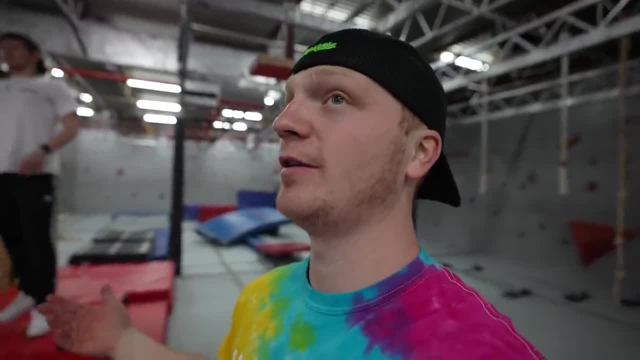 I will give you $100. You as well. I'll give you $100. Thank you. Hang on the bar for 100 seconds and you get $100. So $1 every second that you hang, But if you fall you don't get anything. Yeah, honestly here, let's do this. 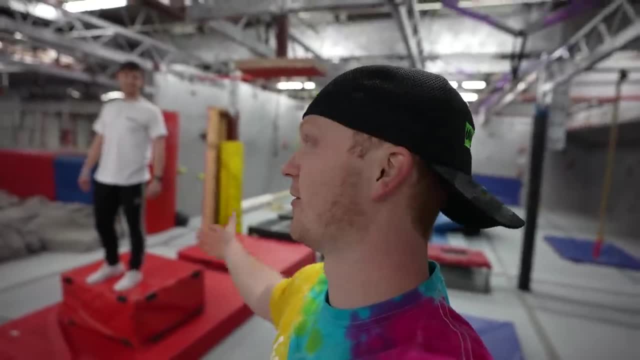 $1 for every second you hang. So if you hang for 200 seconds, I'll give you $200. Okay, If you hang for 1,000 seconds, I'll give you $1,000. 3,, 2,, 1, go. 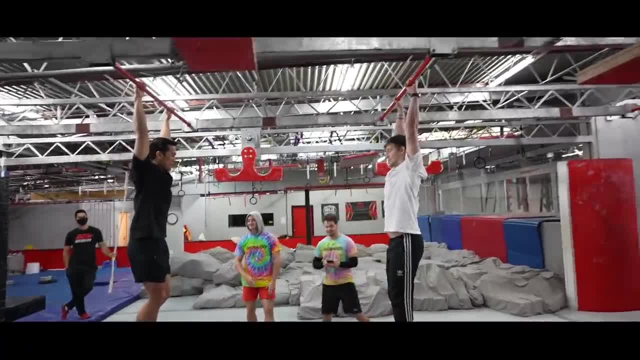 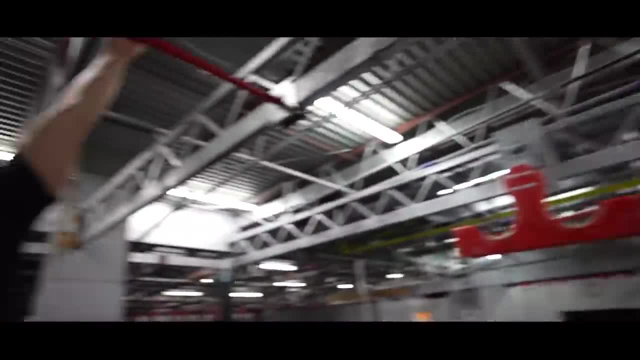 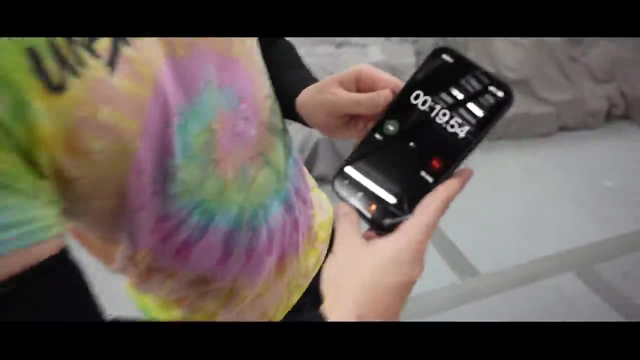 Yeah, move that cheater. Has it been 100 yet? It's only been 8 seconds. 10, 9, 8, Hi. How do you feel I'm tired already, bro? How long has it been 20 seconds, It's literally been 20 seconds. 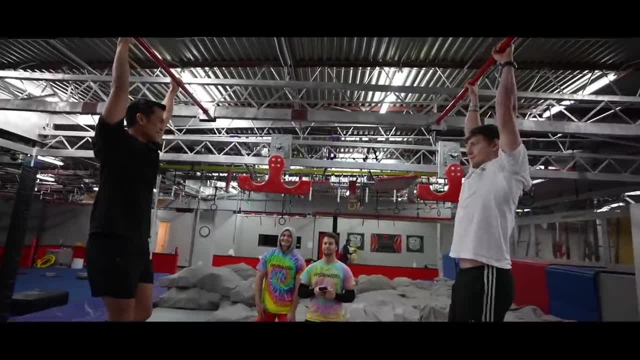 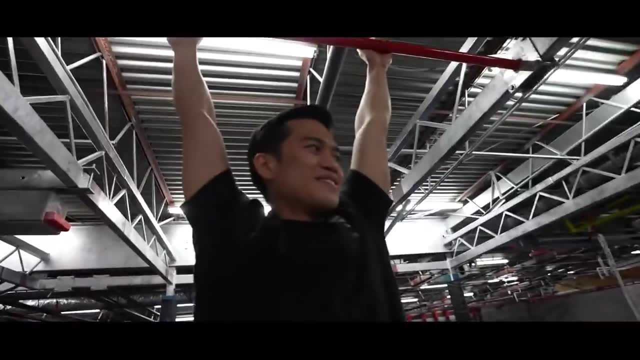 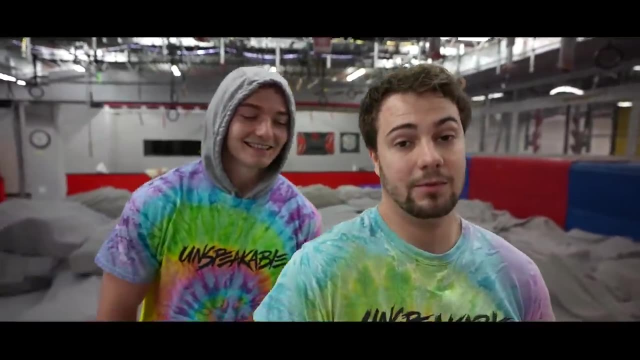 Remember, shake out 35 seconds, I'm gonna make it. Hey, that's a brutal, brutal life. You think they're gonna make it? We'll see 100 seconds. what is that? that's a minute 30? A minute 30. 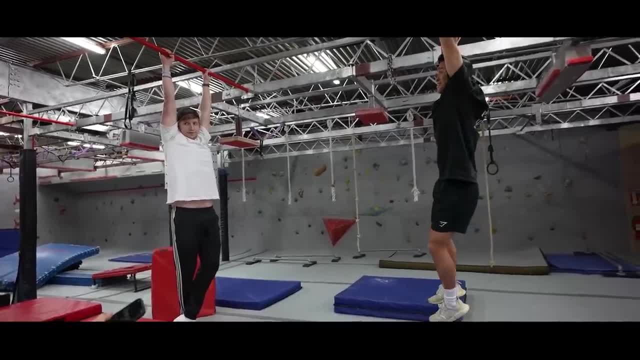 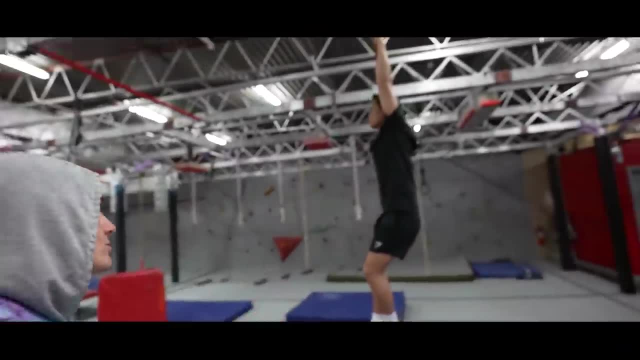 Yeah And Oh. one minute, Cedric can pull up. Well, Jordan has fallen. He fell at 1.04. All right, Cedric, you got this, you got this. Remember everything you sacrificed in life to get to this point. Every second you make it count. 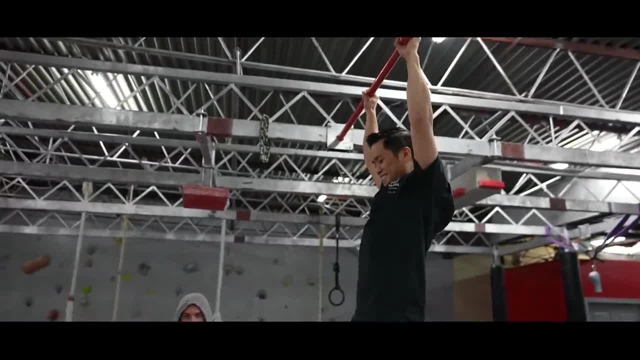 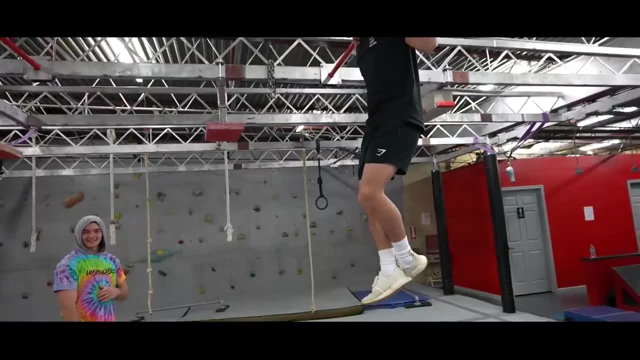 Every second you make it count. Oh, Oh, You decided to show off a little bit. Still is: Wait, what's he got right now? 130, 130, All right, 30 more seconds, No, 10, 140, No, it's 5, A minute 40, something like that.